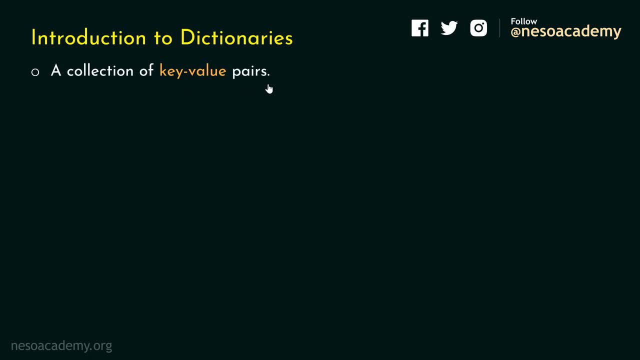 The key in a key-value pair acts as a unique identifier, and a value can be any Python object Dictionaries allow us to store and retrieve values based on their keys, providing a way to map and organize data efficiently, And the syntax is as follows: 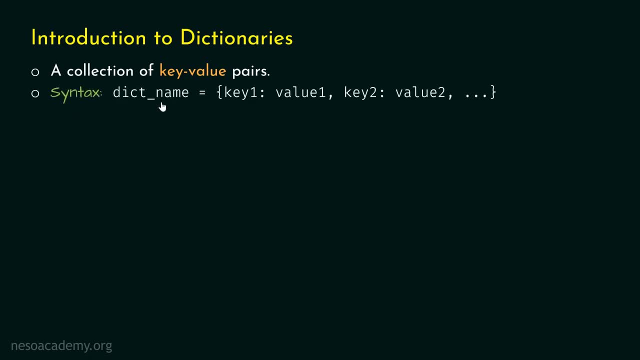 We first need to specify the name of the dictionary. It is represented by dict name, followed by equal sign, which is the assignment operator. Then, within curly braces, we can specify as many key-value pairs as we want, But each key-value pair must be separated by a colon. 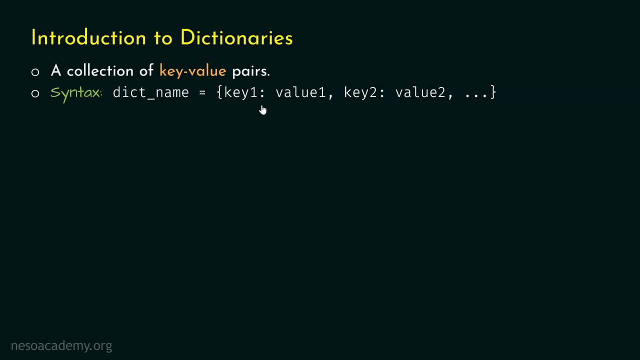 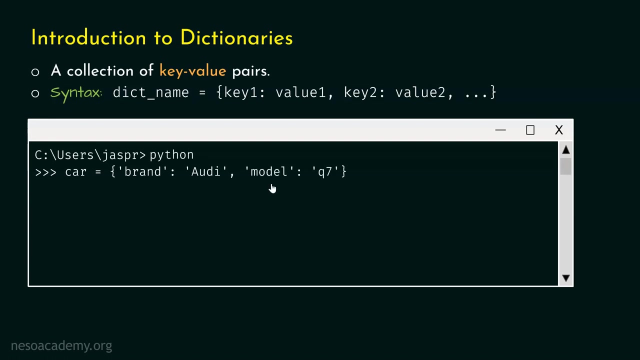 So this is very important. Now let's see how to create a dictionary in Python For this. we will open our command prompt and we will activate the Python interactive shell. Now let's type this command: car equal to brandaudi model q7.. 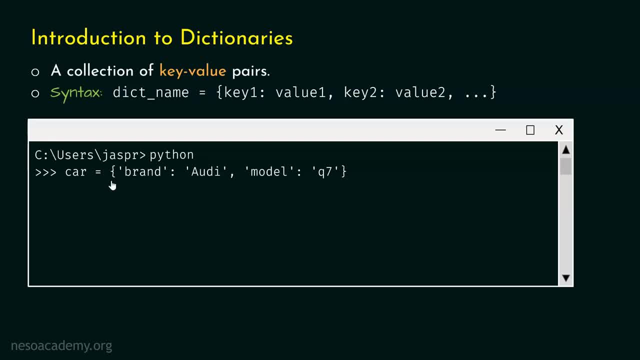 We are trying to model a car through this dictionary. In this dictionary we have a total of two key-value pairs. The first key-value pair is brandaudi and the second key-value pair is model q7.. Each key-value pair is separated by a colon. as it can be observed, 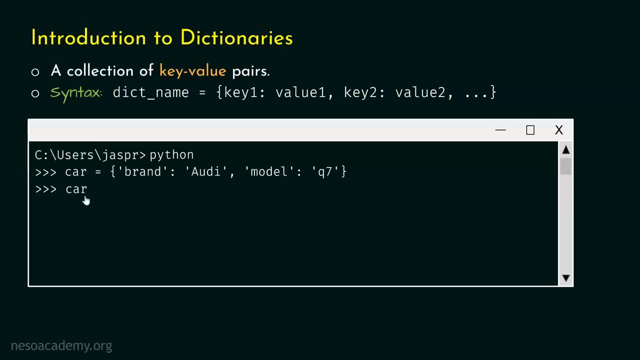 Now let's hit enter and type car, and now to see the dictionary, let's hit enter again. We will get the dictionary with two key-value pairs: brandaudi and model q7.. I hope it is clear how to create a dictionary in Python. 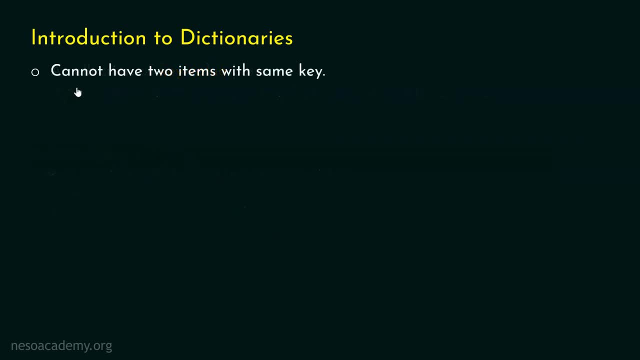 Now let's move on to the next point. A dictionary cannot have two items with same key. This means that duplicates are not allowed in a dictionary. If we try to store duplicates in a dictionary, let's say we decided to store two items with 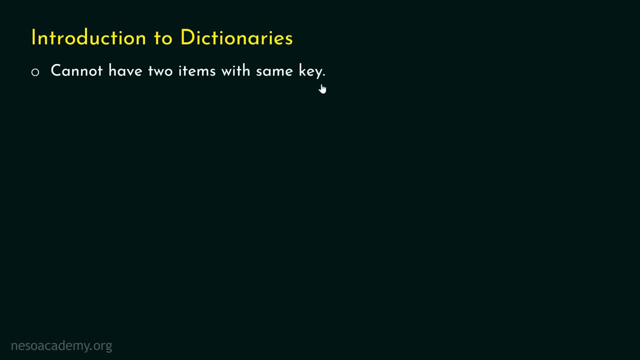 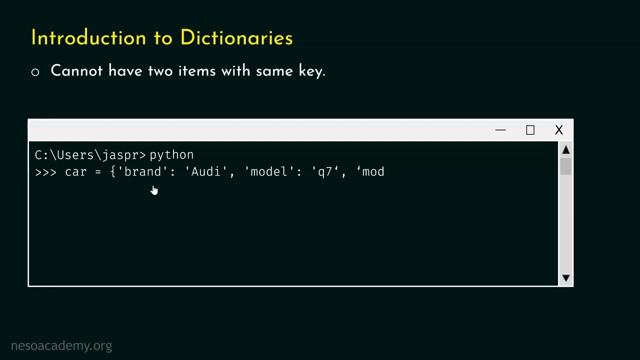 same keys, then only one item will be stored in that case. So which item, Which item will be stored? Let's see with the help of an example. Let's open our command prompt once again. Let's create a new dictionary car with three key-value pairs: brandaudi, model q7 and model. 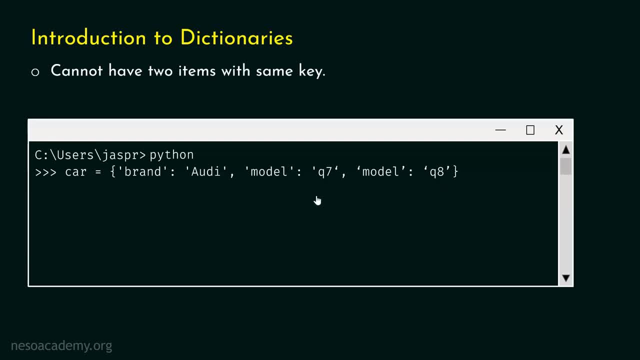 q8.. As it can be observed, we are trying to duplicate an item: Here we have model q7 and here we have model q8, which is not allowed, Although we will not get any error message, But only one item will be stored inside this dictionary. 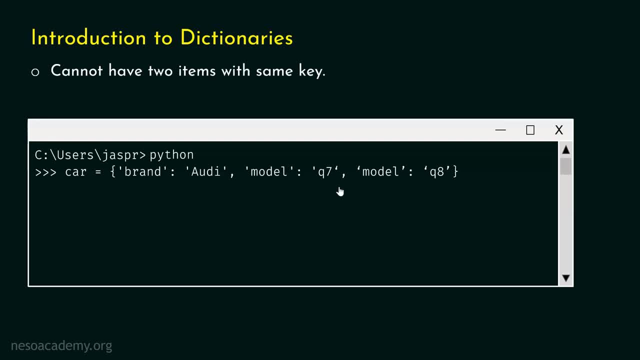 Either model q7 will be stored or model q8.. Now the question is which key-value pair will be stored inside the dictionary, The one which comes later? So this key-value pair will be stored inside the dictionary. Now let's hit enter and type car, and let's again hit enter. we will get this dictionary. 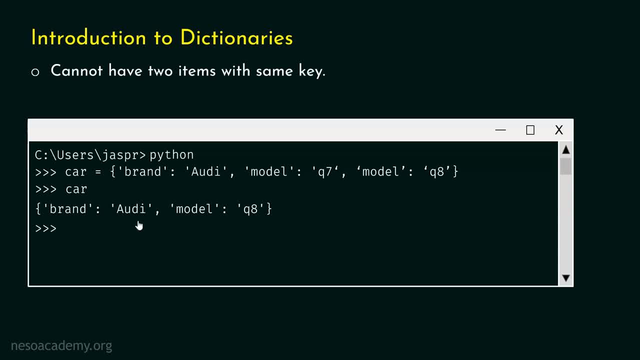 with a total of two key-values: Brandaudi and model q8.. We were trying to store duplicates, but we are only getting one key-value pair. You must always remember that the key-value pair which comes later will always be available in the dictionary. 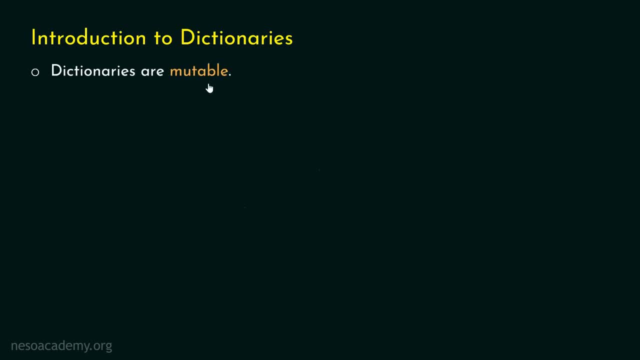 Now let's move on to the next point. Dictionaries are mutable, which means that dictionaries are changeable. We can change value of a specific key By referring that key. Let's see how to do this. In order to understand this, let's consider the same car dictionary which we have considered. 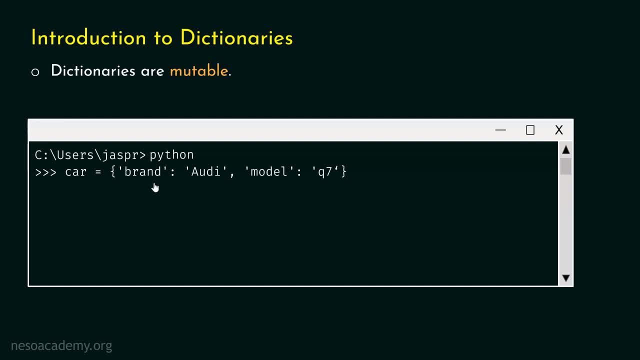 in the first example, That is car equal to brandaudi and model q7. Let's hit enter and now let's type car model equal to q8. Here we are trying to update this value. to this value We want to change q7 to q8.. 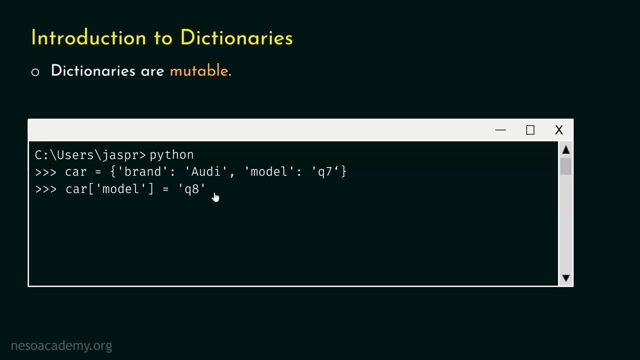 For this, we need to change the value to q8.. For this, we can refer the key model like this, within square brackets, and with the help of this assignment operator, we can update this value q7 to q8.. Now let's see what happens when we try to print this dictionary. 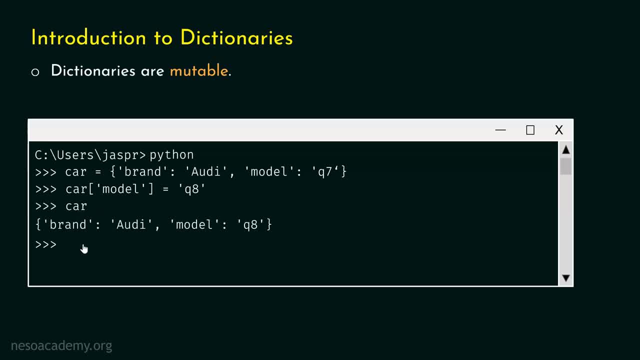 Let's hit enter and type car and let's again hit enter, We will get this dictionary where we can observe that model is now updated to q8.. So with this I hope it is clear How to update any item. Let's see what happens when we try to update any item in a dictionary. 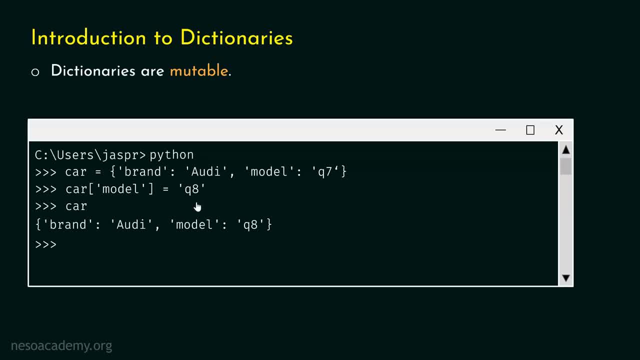 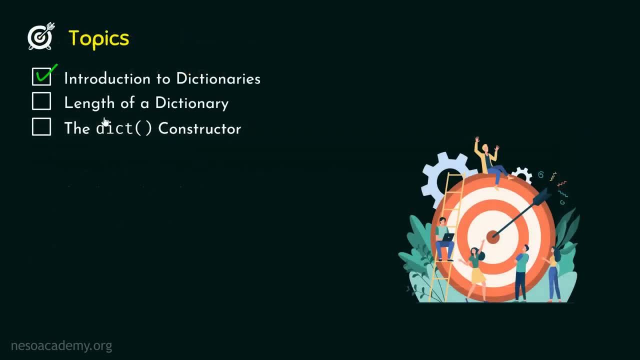 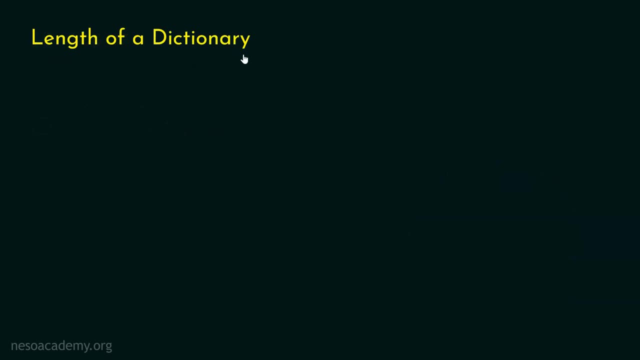 So dictionaries are mutable. We can make changes to any value in a dictionary. Now, with this, we are done with the introduction to dictionaries. Let's move on to the next topic, that is, length of a dictionary. So how to determine the length of a dictionary? 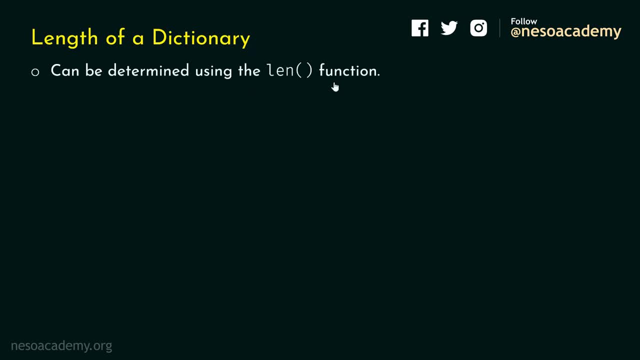 The length of a dictionary can be determined using the len function. Also, we must note that It gives the count of key value points. So let's see how to do this. Let's open our command prompt and let's consider the same car dictionary with brand Audi and model q7.. 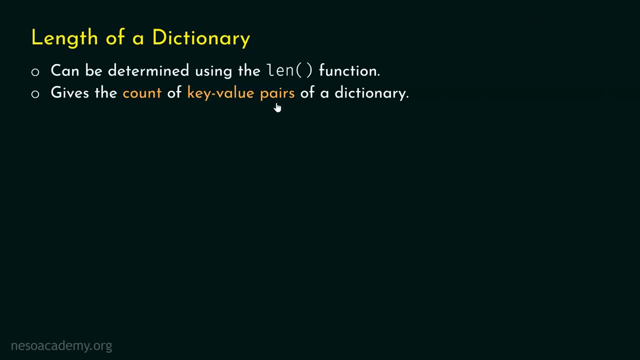 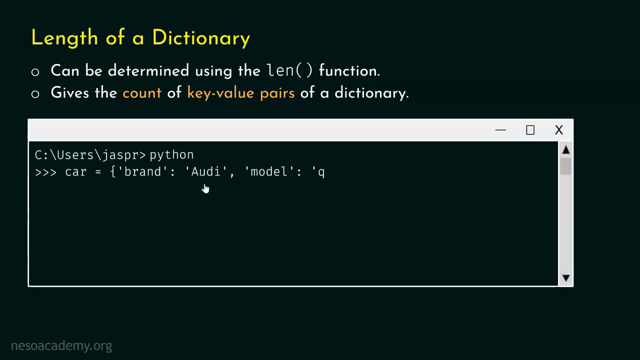 It will always give count of pairs, not individual keys and values. Let's open our command prompt and let's consider the same car dictionary with brand Audi and model q7.. Now let's hit enter and let's calculate the length of this dictionary by providing the name of this dictionary to len function. 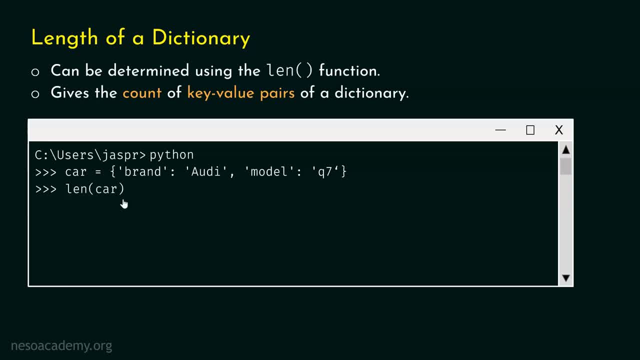 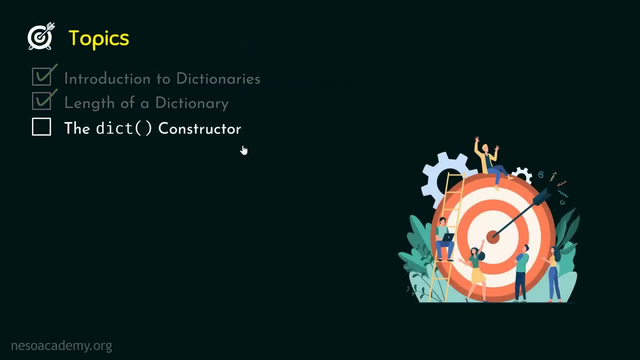 Let's do this: Let's type len car, Let's hit enter. We will get two as the result, because there are two key value pairs in this dictionary. I hope this is clear. Now let's move on to the next topic, that is, the dict constructor. 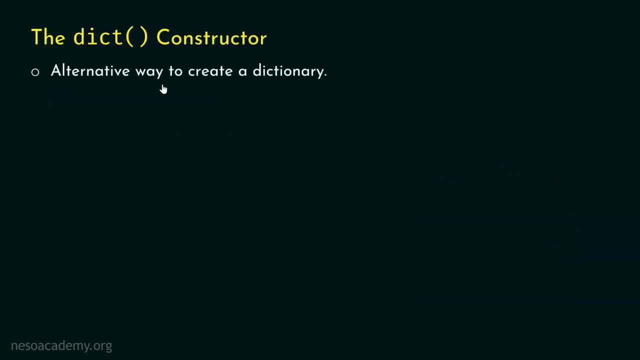 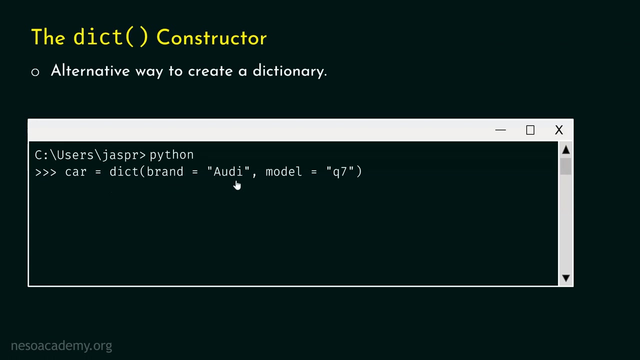 The dict constructor provides an alternative way to create a dictionary. We know one way to create a dictionary. Now let's try to create the same car dictionary with brand Audi and model q8. With the help of this dict constructor. For this, let's open our command prompt and let's type: car equal to dict, brand equal to Audi. comma model equal to q7.. 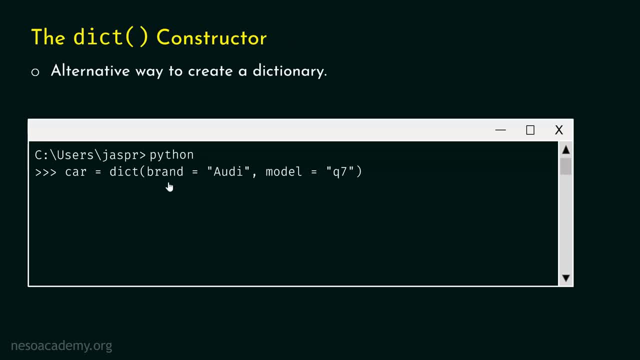 Note that here keys are not wrapped within single or double quotes. Also, in place of columns we have equal signs. Now let's hit enter and type car and let's again hit enter. We will get the same dictionary with two key value pairs: brand Audi and model q7. 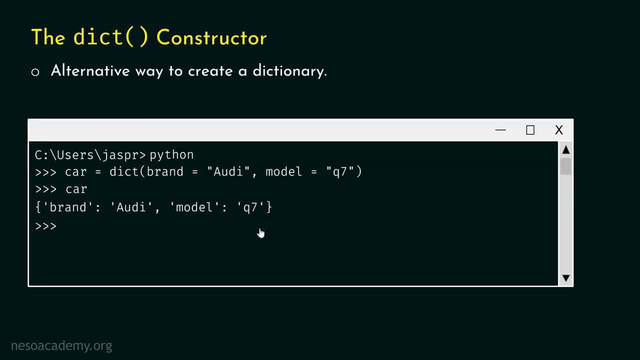 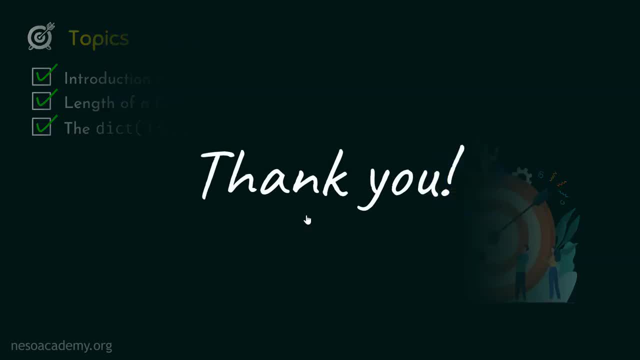 So it is up to you which method you want to use to create a dictionary. I hope with this all the topics are clear. Okay, friends, this is it for now. Thank you for watching this presentation. I will see you in the next one. Bye, bye.